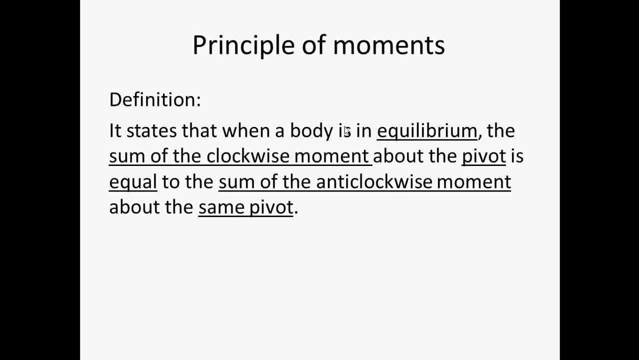 You cannot leave any of these keywords out, because they will not make sense if any of these keywords are missing. So, in order to understand the principle of moment, let us look at a case where you have only one force acting on a seesaw. 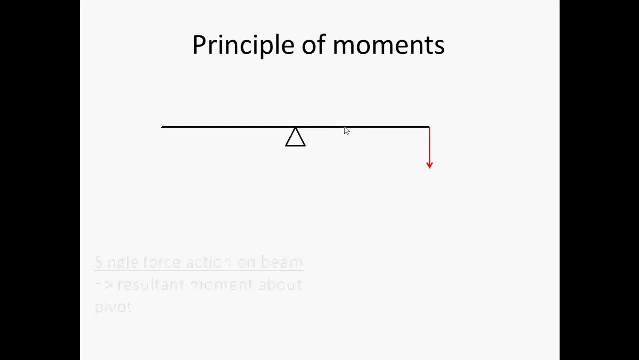 Now, if you have only one force acting on a seesaw, obviously there will be a resultant moment about the pivot. Okay, what will happen? Okay, obviously the seesaw. of course it can't rotate so much, but 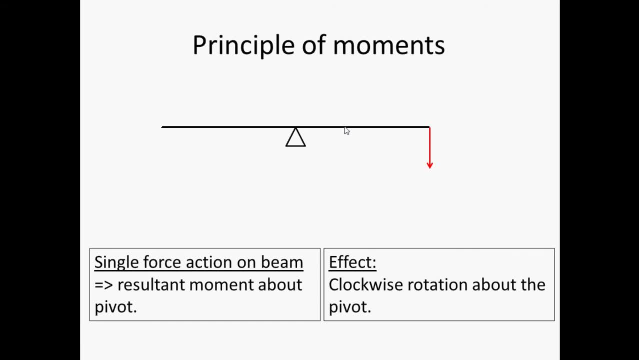 the seesaw will basically rotate in a clockwise direction. If it can, it probably will rotate the full circle, Alright. So that is how what will happen if there is resultant moment? But what happens if you have an equal force placed at an equal distance away at the opposite side of the seesaw? 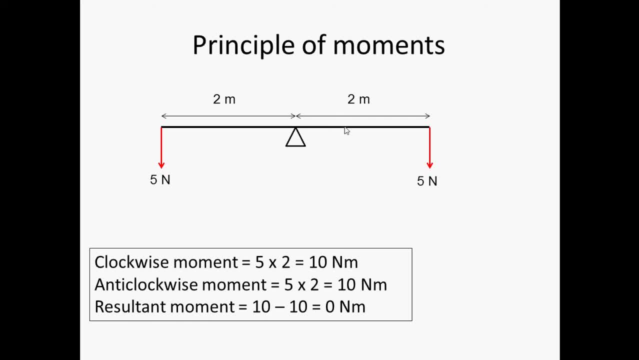 What will happen Now? if you do a calculation, you will realize that the clockwise moment is 5 times 2.. The anticlockwise moment is also 5 times 2.. So if you subtract these two moments, because they are in the opposite direction, you get 0 Nm. 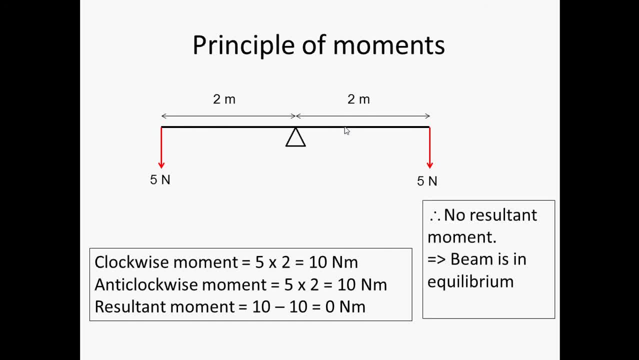 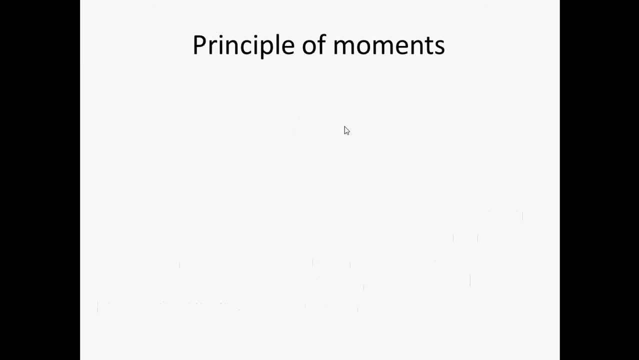 So it means that there is no resultant moment and because of that the beam is at rest or in equilibrium. Okay, So when the beam is in equilibrium, we know that the clockwise moment minus the anticlockwise moment equal. 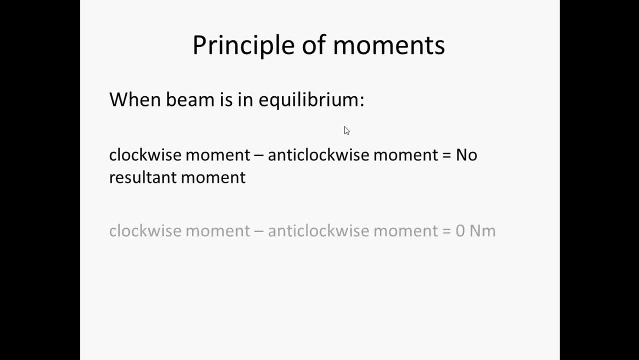 equals no resultant force. So in that case the clockwise moment minus anticlockwise moment equals 0.. Okay, The Nm is just a unit. So if you rearrange the formula, you have your principle of moments. The principle of moments states that the clockwise moment equal to the anticlockwise moment. 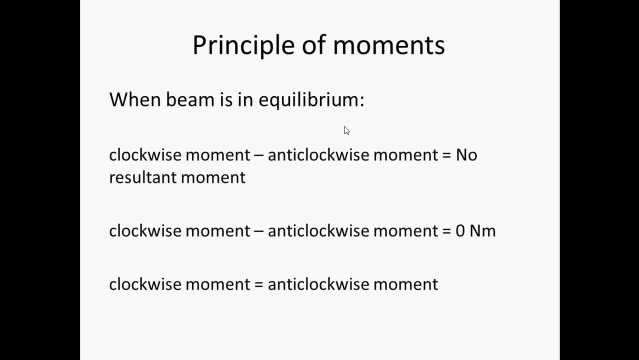 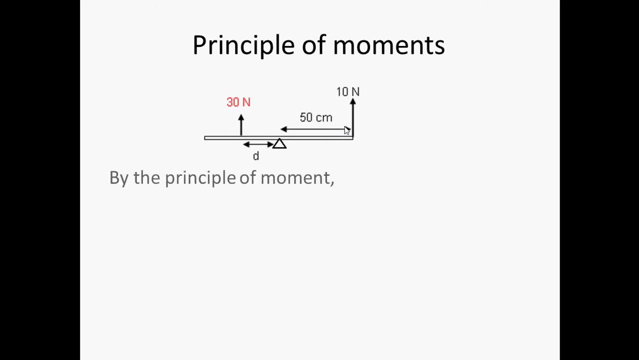 about the same pivot when in equilibrium. Alright, So that's how it arises, How the principle of moments arises. So let us deal with principle of moments by doing a few examples. Now look at this question. Okay, If you are trying to solve any principle of moment question, you must write down the statement. 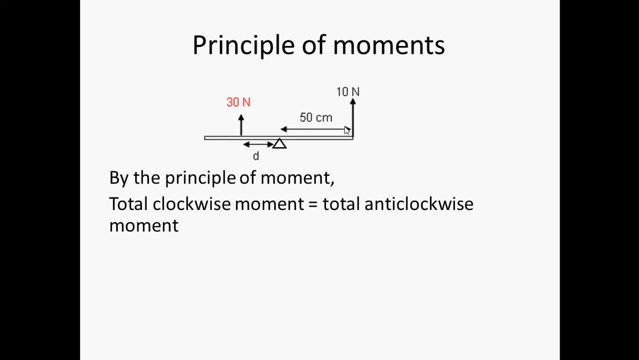 You must write down by the principle of moment. total clockwise moment equal to total anticlockwise moment. So if this question is asking you to find the unknown D, such that the beam is balanced, Alright, You will find. So the total clockwise moment will be what? 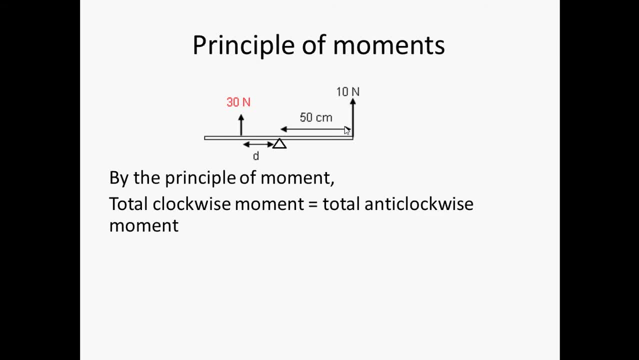 The total clockwise moment will be: Okay, let me just turn on my pen. Okay, The total clockwise moment will definitely be this guy here, which is 30 times D, And the total anticlockwise moment will be this one here, which is 10 times 50.. 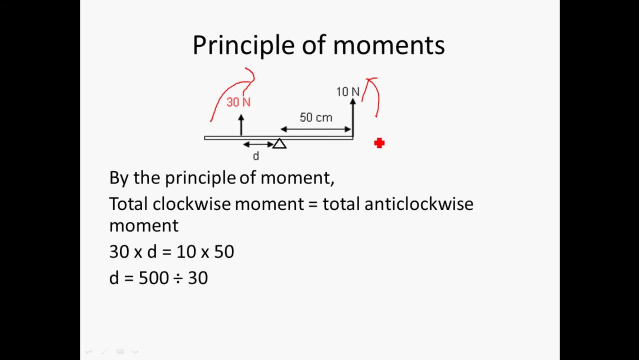 Right. So because of that, if you solve it, you get 16.7.. So that is the answer. Because this moment must balance this moment for the principle of moment to exist. That's why, For the principle of moment to be true, 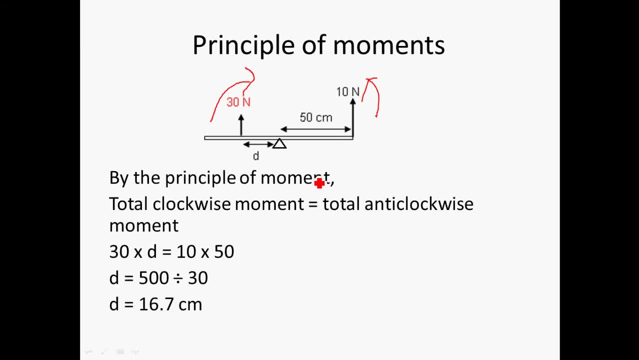 That's why the unknown D is equal to 16.7.. You can solve it by using equation. Now, second example: What if, in this case, There are more than one force? There are two forces here and one F here. 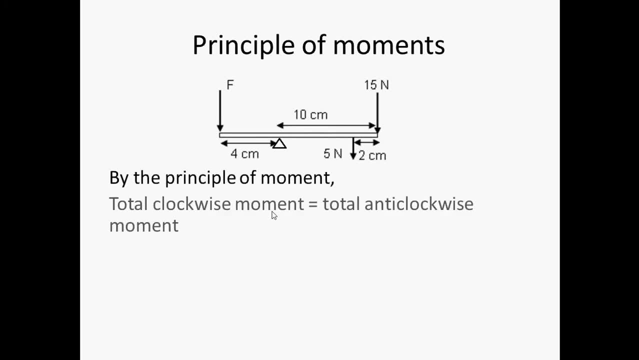 So how do you find the unknown F In the same way? first of all, you need to write down the statement. After you've written down the statement, okay, you know that this 15 N and this 5 N, both are clockwise moment. 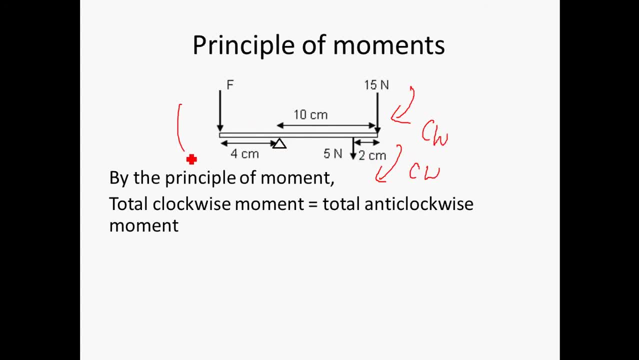 Right, So you have two clockwise moment and one anticlockwise moment. So you need to sum up. You need to sum up all the clockwise and all the anticlockwise moment. So the clockwise moment will be 5 times 10 minus 2.. 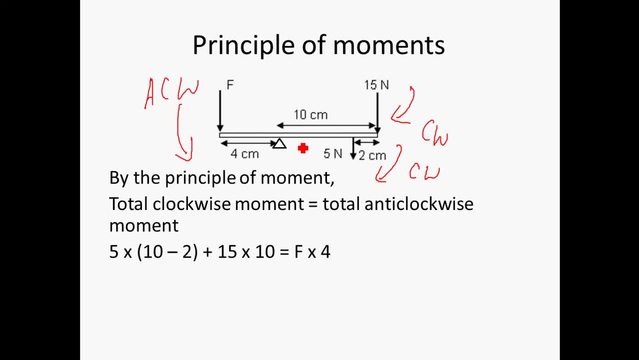 Then you say: why is it 10 minus 2?? Remember the distance D has to be the perpendicular distance from the force to the pivot. So it has to be this distance, which is 10 minus 2 or 8 cm. 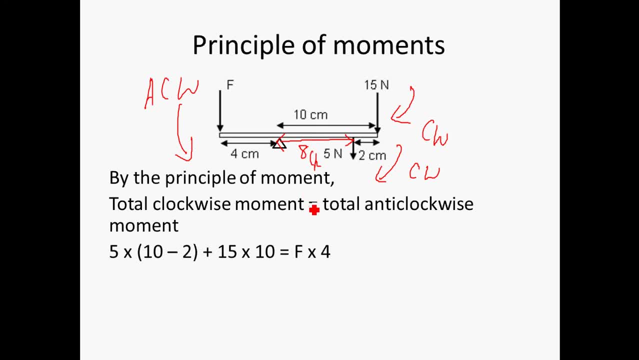 So this is 8 cm plus 15 times 10.. Alright, So this is the sum of two moments Equal to 5 times 4.. So you'll get 47.5.. Okay, So let's move on to the next one. 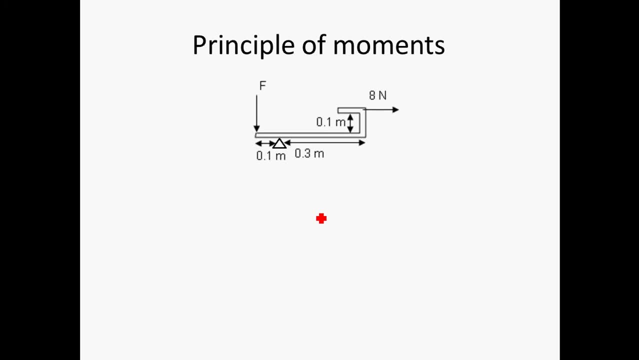 How about this case? You have a body that is very strange shape. Does it matter whether the shape is strange or not? It doesn't matter. The principle of moment will still apply, But in this case you need to be very careful. 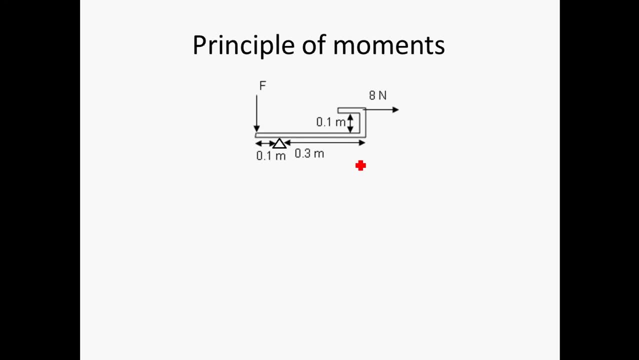 You need to identify which one is your clockwise and which one is your anticlockwise. Now for this one. obviously, this will be your anticlockwise Right, But this one is harder to see. How do you know this is clockwise. 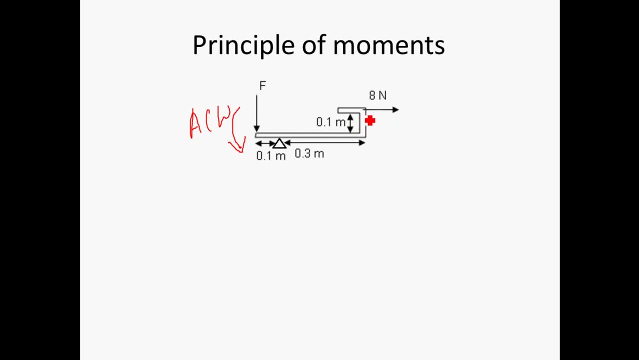 Okay, although this force is acting in this direction, if you just imagine pulling this rigid L-shaped thing in this direction- it will still rotate downwards. So because of that, this is still a clockwise moment. Now the only hard part is that for this 8 N force, 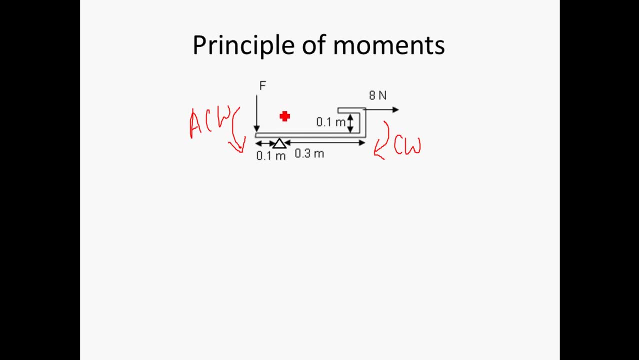 what is the perpendicular distance? Okay, Remember your first video: Always extend your force, the line of action of your force, and then draw your perpendicular distance. So this will be your perpendicular distance And because this distance is the same as 0.1, you can use 0.1 directly. 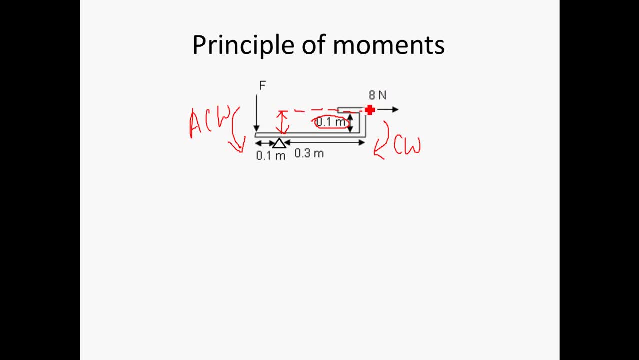 Alright, So this will be your perpendicular distance for the 8 N force to the pivot. So, writing the statement down again, your clockwise moment will be 8 times 0.1.. Your anticlockwise moment will also be F times 0.1.. 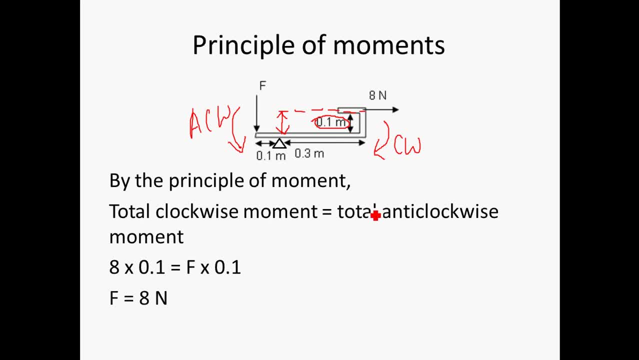 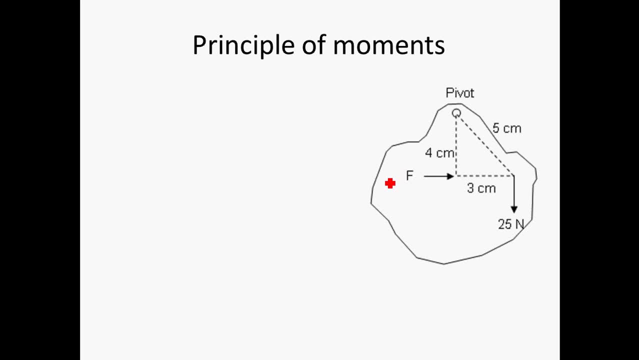 So F is obviously 8 N. Alright, So let's look at this question. Alright, I think probably it's the last question already. Okay, how do you find the unknown force F if it is balanced? Okay, so in this case it's a little bit more complicated. 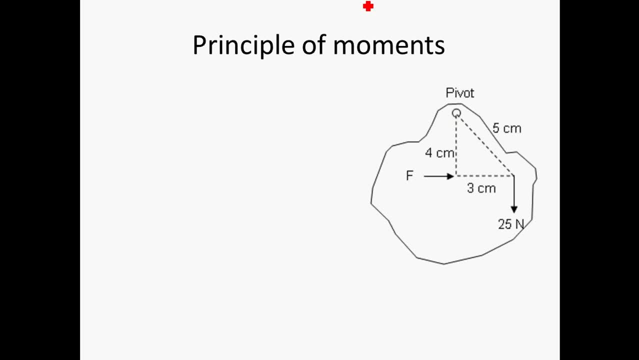 Again, you need to be careful. You need to find the perpendicular distance. So first of all also, you need to know which one is clockwise and anticlockwise. This will be your clockwise moment. Why? Because this is a rigid body and you're pulling the rigid body down in this direction. 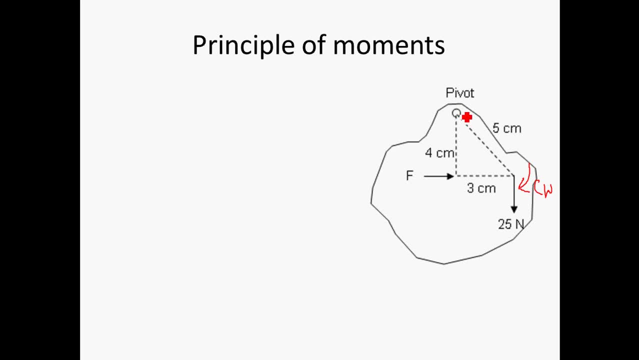 with the rigid body pivoted here. So imagine this is a disc and then you pull at this point. Alright, Obviously it's going to rotate clockwise. Now if you have an F that's in the center and you're pushing in this direction,